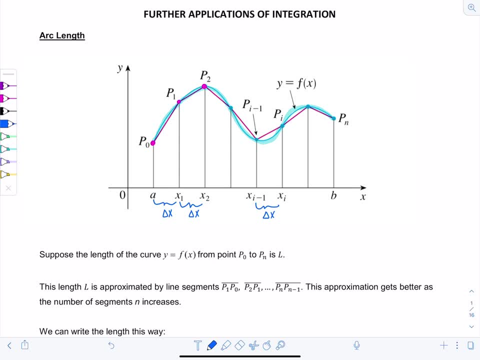 with the actual length of the curve, And so, in order to improve our approximation, we can just take more and more line segments. we could let n get larger and larger and chop it up into tinier bits. that way there's less error. Well, I mean, we're in calculus, so why stop at a finite number? Let's just let n go to infinity. 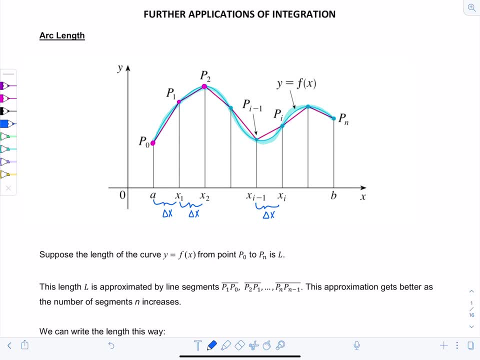 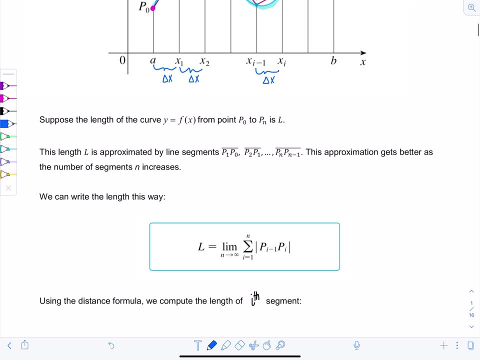 let's have infinitely many little line segments, and then our error will approach zero. and that's precisely where the formula for arc length comes from. So we can write it in the following form: the limit as n' approaches infinity of the sum, and these are all the little line segments. This is some arbitrary. 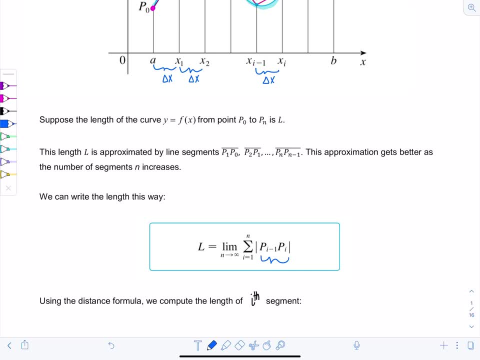 ith line segments. so we're summing them all up, from i equals one to n and we're taking the length of each of those. Okay, now, using the distance formula, like I mentioned earlier, we can compute the length of the ith segment. Remember to use the distance formula. we need to know what the 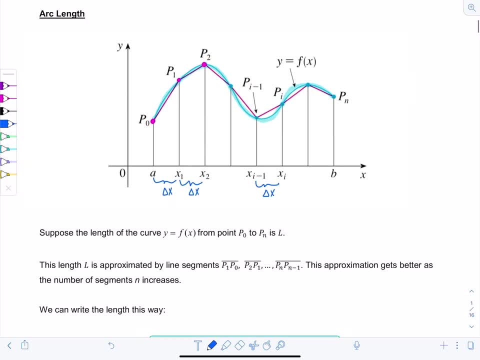 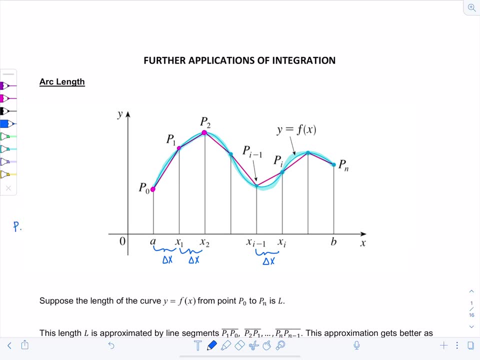 coordinates are for each of those points. So let's go back to the graph. here we're working with the ith line segment. I want to know what the coordinates are for p sub i minus one and p sub i. So p sub i minus one. can you see where it is? it's right. here it's x coordinate is x sub i minus one and the y coordinate would be y sub i minus one also, and similarly p sub i has coordinates x sub i, y sub i. can you see that here? x sub i, and then it would be the y value there. 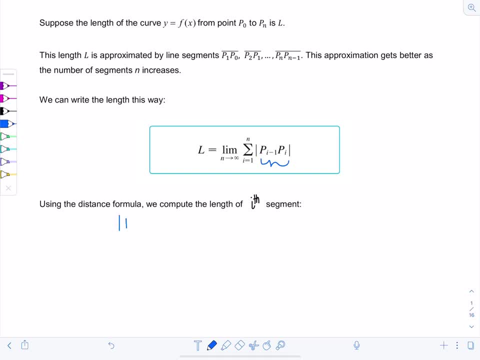 Okay, so let's put this all together. So that means the length or magnitude of line segment p sub i minus one to p sub i. this here is equal to the square root of: I have x sub i minus x sub i minus one squared, plus y sub i minus y sub i, minus one squared. 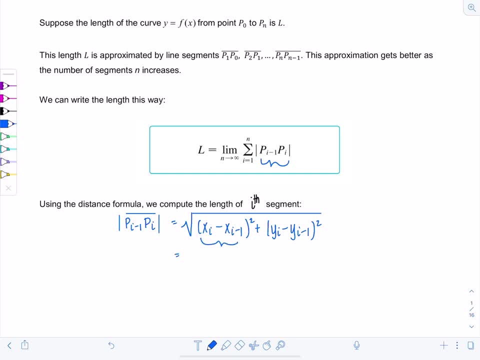 All right, and then notice x sub i minus x sub i minus one, that's just delta x. Right, we chopped up the interval from a to b into n many pieces evenly. Now can I replace y sub i minus y sub i minus y sub i minus one with delta y. 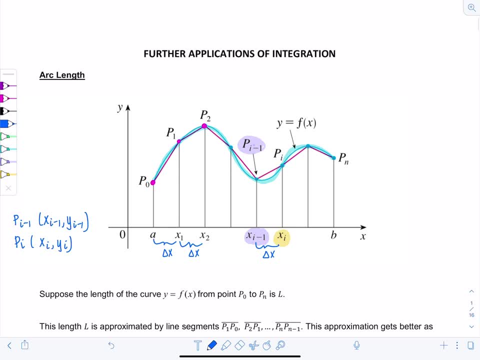 No, not quite. look back at the graph. notice. delta x is consistent, right for all of our partitions. We evenly spaced them, We spaced them out. but delta y is not the same for every interval. here delta y is large, here not so large. here it's negative, a little more negative. so delta y depends on i, it depends. 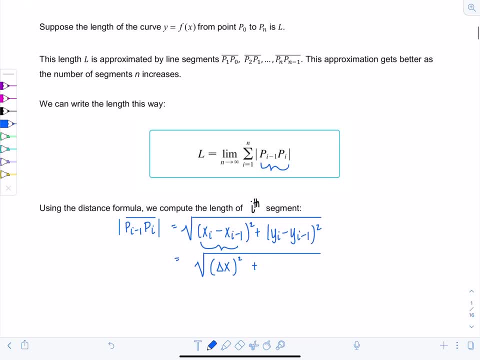 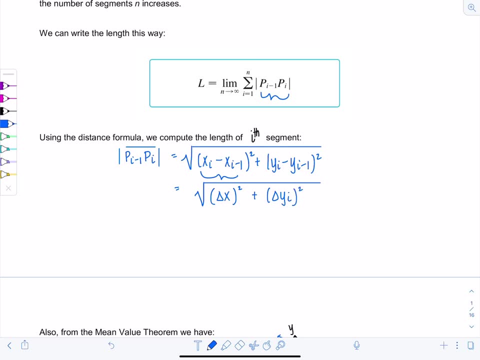 on which partition you're in. so what I'm going to mark it or replace it with is a delta y sub i squared, since that one's changing. Okay, we're going to put this portion on hold, And then we're going to use the mean value theorem now to help us proceed with getting. 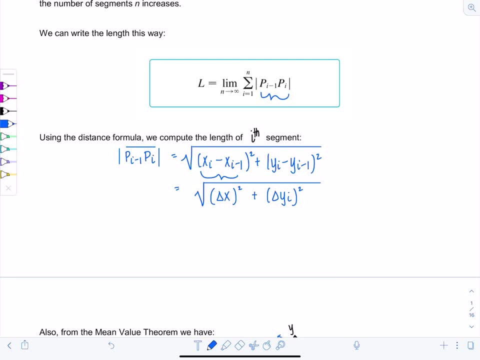 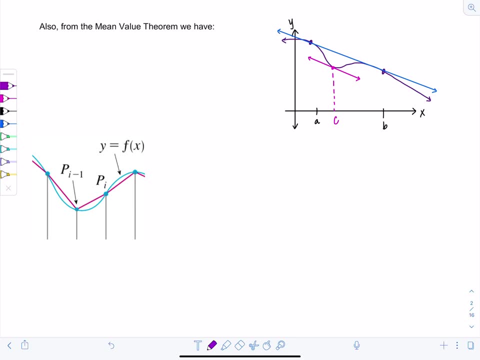 the formula for arc length. Do you remember the mean value theorem back from your calculus one days? well, remember. the mean value theorem tells us, as long as f is continuous and all that good stuff, that on the interval from a to b we can find some f prime of c that is going to equal f of b. 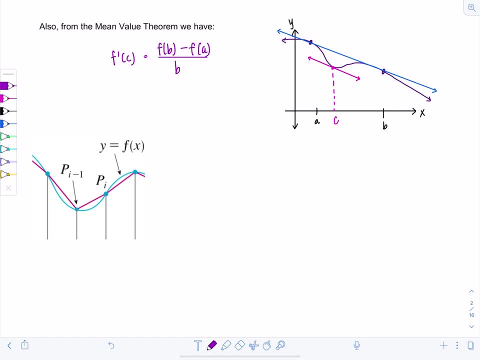 minus f of a over b minus a, and just remember this graph. it'll help you understand the mean value theorem. The right hand side that I've written here gives us the slope of the secant line that goes through the function y equals f of x, which is shown here. 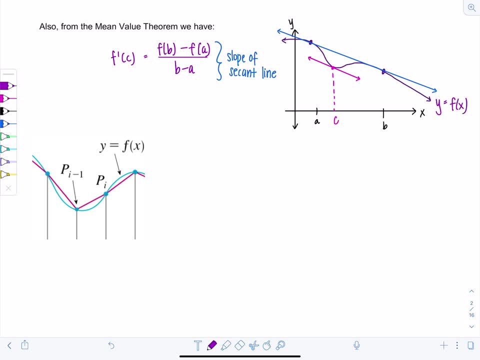 This is y equals f of x. notice: the blue line gives us the slope of the secant line, change in y over change in x, and the mean value theorem tells us that we can find some c, that's on the interval from a to b, where the slope of the secant line is going to equal the slope. 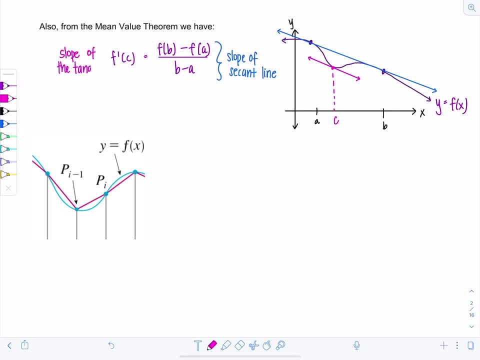 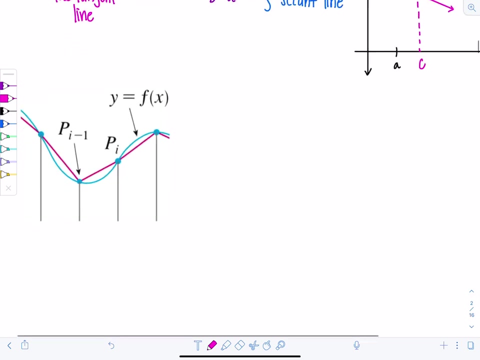 of the tangent line. Let's see, I notice they're parallel, right, okay, why am I bringing this up? well, look at what's going on at each of these little partitions to our curve. I'm going to focus in right now on the i-th subinterval, and here we have a secant line. oh, yes, we do. this is the secant. 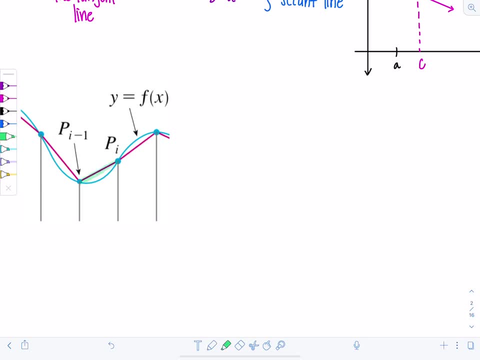 line right here from p sub i minus a to b. I'm going to focus in right now on the i-th sub i minus one to p sub i. could we get the slope of that secant line? well, remember, slope is change in y over, change in x, change in. 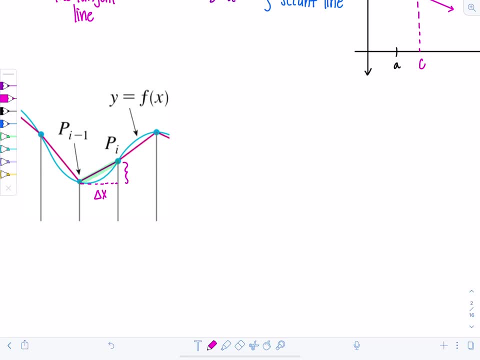 x, I know, is delta x. change in y is going to be delta y sub i and by the mean value theorem, I know I'm going to be able to find some point. normally we call it c. I'm going to call it x sub i star. 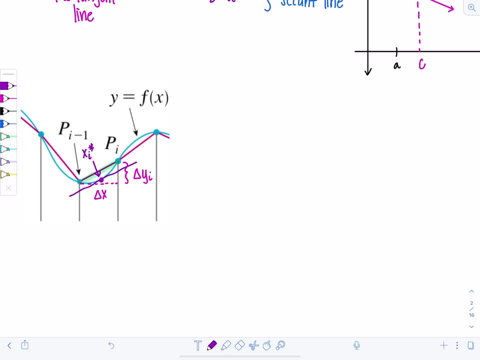 I'm going to call it x sub i star. I'm going to call it x sub i star. So that means that the slope of the tangent line is equal to the slope of that secant line. so that purple line I just drew has the same slope as that little line segment. 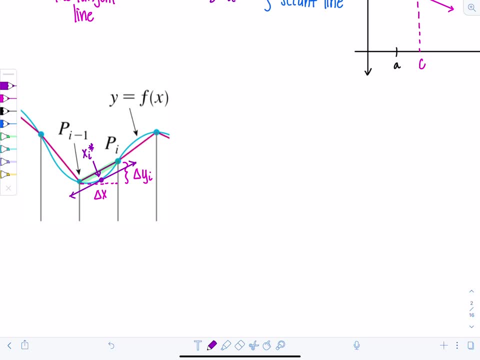 from p sub i minus 1 to p sub i, and I know I can do this at every sub interval on this curve because of the mean value theorem. so that means f prime of x sub i star is going to equal. remember this is the slope of the tangent line. it's going to equal the slope of the secant. 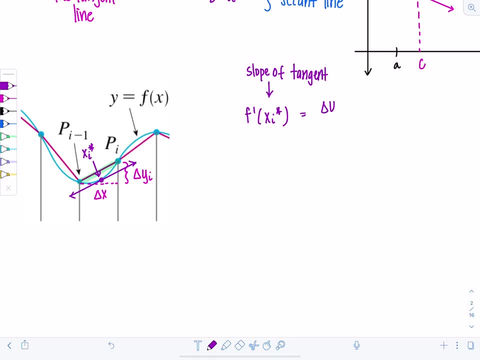 line or line segment which is rise over, run. delta y sub i over delta x. This is slope of the line segment. But what was the point of this? Well, now I can rewrite: delta y sub i equals f prime of x sub i star times delta x. Ooh wonderful. Now I'm going to put this back into the distance. 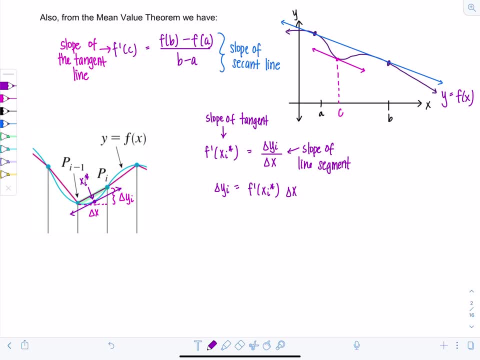 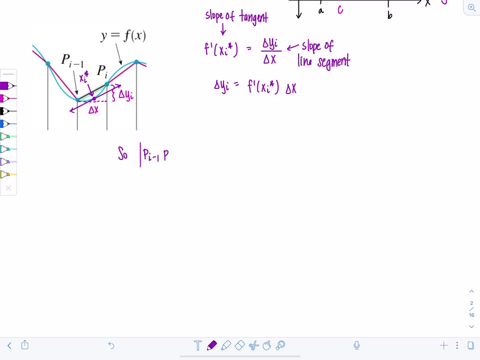 formula where I was finding the length of each of those little line segments. So, revisiting, I know the length of segment p sub i minus 1 to p sub i is equal to square root. And then remember we had delta x squared plus delta y sub i. 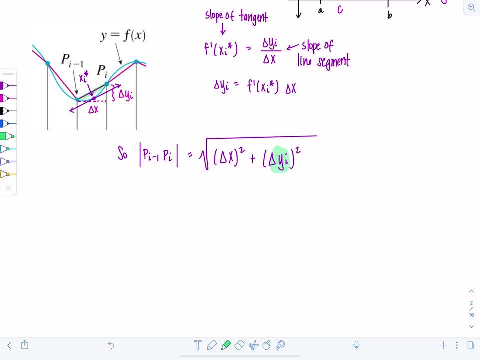 squared. And then now I'm going to replace delta y, sub i squared with this expression here: f prime of x, sub i star times, delta x. Here we go. Exciting stuff, people. So this is delta x squared plus f prime of x, sub i star. delta x squared. 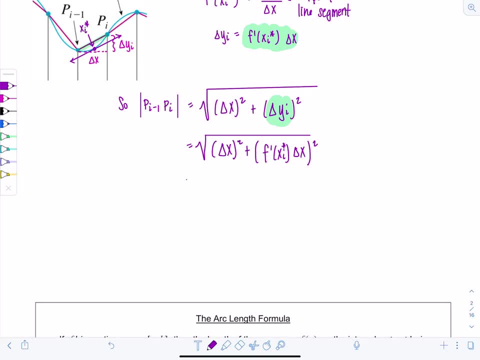 Okay, I can factor out a delta x squared from the expression. So I have delta x squared times 1 plus f- prime of x sub i star. That's still squared, though, And then I'm left with square root: 1 plus f- prime of x sub i star. 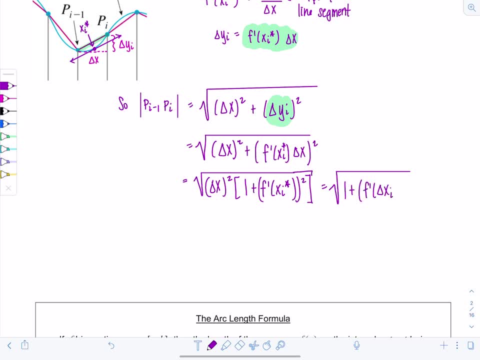 So I'm going to take this f prime of x sub i star plus f prime delta x. Oh, no, delta, excuse me, Just x sub i star. This is all squared times. and then that delta x squared, I can pull it outside of the radical. 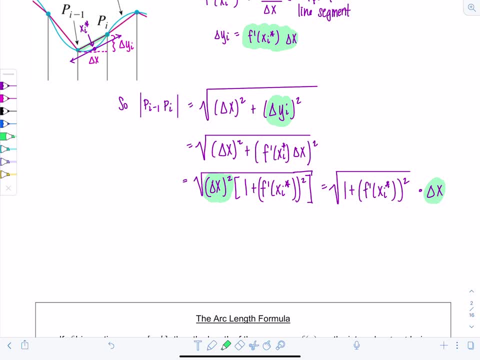 And now it's just regular delta, x, Woo. So I'm going to replace this in that original formula. Remember we had that the arc length was equal to the limit, as n approaches infinity, of the sum, i equals one to n. And then, instead of writing the length, 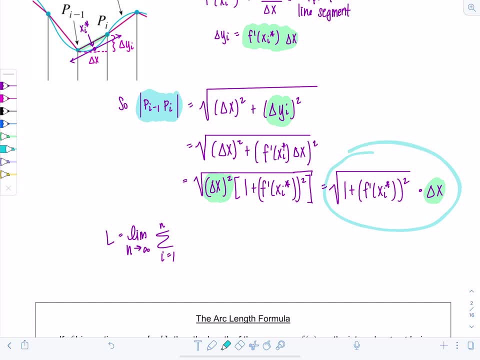 of p sub i minus one to p sub i. now I have this expression here, So this is gonna be square root of one plus. let me switch to brackets, it'll look so clean. f: prime of x sub i. star squared times, delta x. 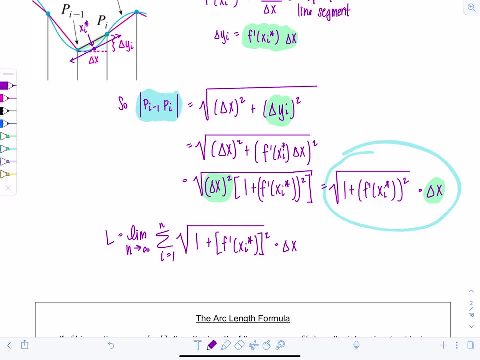 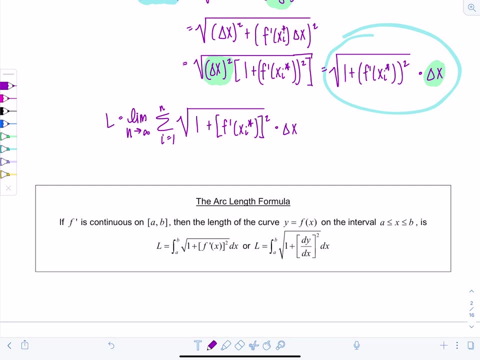 Well, I see a limit, as n goes to infinity, and a sum that means we are gonna integrate. oh yes, And here's your arc length formula. So if f prime is continuous on a to b, we need that because, remember, we used the mean value theorem. 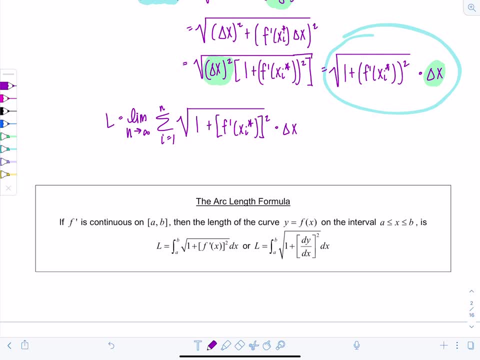 to get this formula. then the length of the curve y equals f of x on the interval from a to b is given by the definite integral from a to b of the square root of one plus f. prime of x squared dx. All right, such fun. 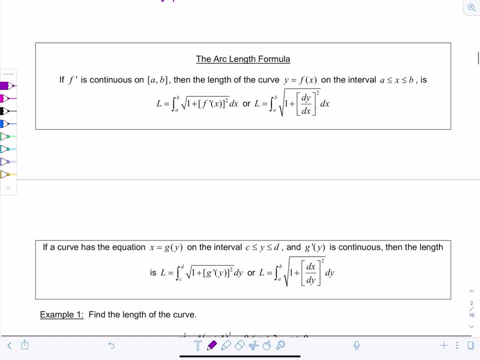 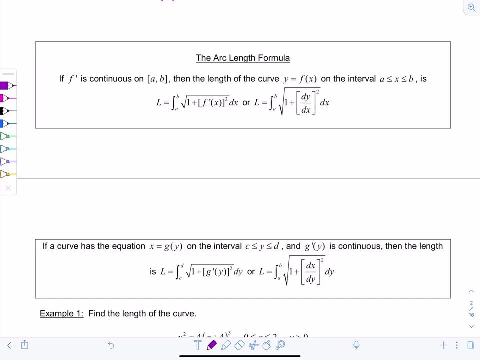 Now, if the curve has the equation x equals g of y, so if it's a function of y on the interval from c to d and g prime of y is continuous, then the length would be the definite integral from c to d of the square root. 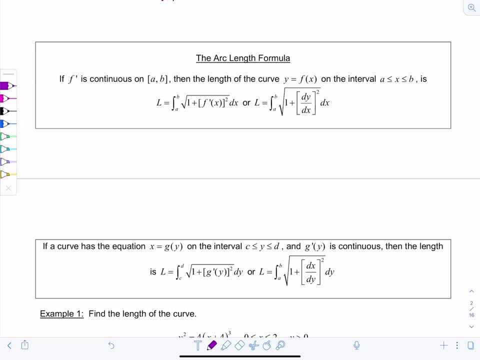 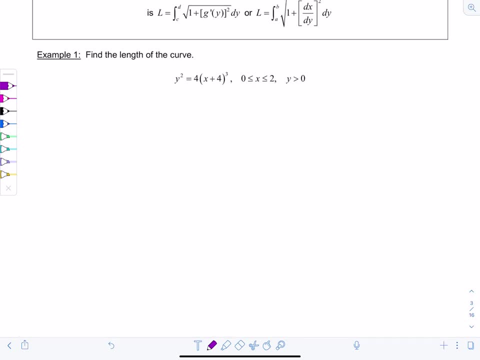 of one plus g, prime of y squared dy. So let's try one out. eh, Here we go And find the length of the curve We have. y squared equals four times x plus four cubed on the interval from zero to two. 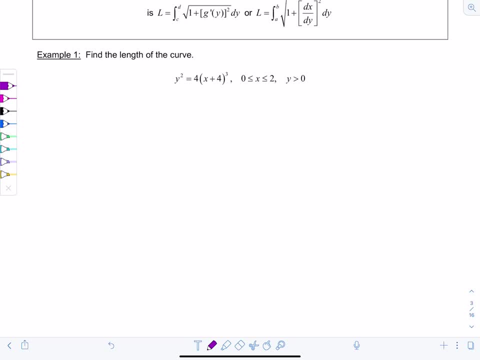 And they're telling us PS y is greater than zero. Okay, so to get started, let's solve for y. So y equals plus or minus the square root of four times x plus four cubed, And I know I'm gonna choose the positive radical. 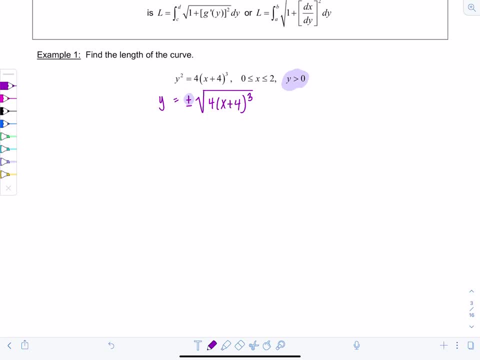 because they told me we're interested only in the portion of the curve where y is greater than zero. So that means y equals two times x plus four to the three halves, if I take the square root of everything. Now, what I like to do is all my prep work ahead of time. 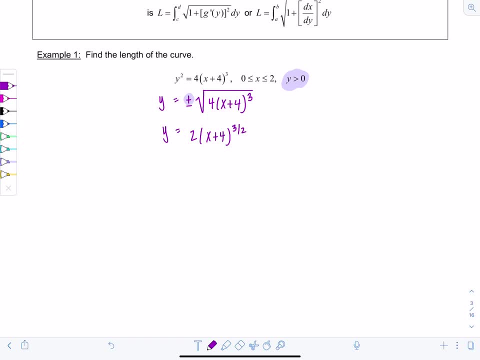 meaning I'm not gonna write out the full integral yet. I'm gonna figure out what f prime is, square it, add one and get that all clean and pretty before I actually write up a full integral. okay, So here we go. f prime of x or dy dx. 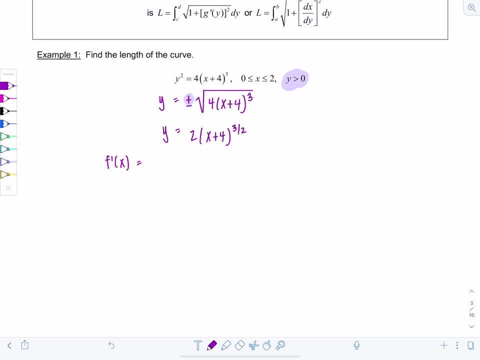 Okay, So f is gonna equal, so I have two times. I'm gonna multiply by three halves. leave x plus four alone, subtract one from the exponent, So it's gonna be one half And we end up with three times x plus four to the one half. 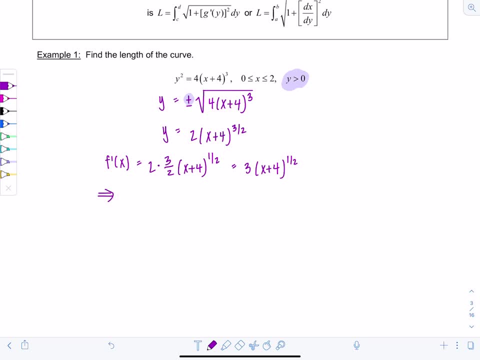 Okay now remember the integrand was one plus f prime of x squared, So let's get that all ready to go. It'll make life easier. So we're gonna have one plus f prime of x squared. Okay, So f prime of x is three times x plus four to the one half. 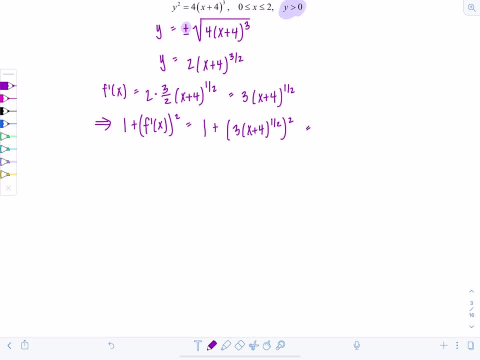 And then we're squaring that, which means I'm gonna have one plus. now be careful: this is nine times the quantity x plus four. If I distribute the nine, that's gonna be nine x plus 36 plus one. So this is nine x plus 37.. 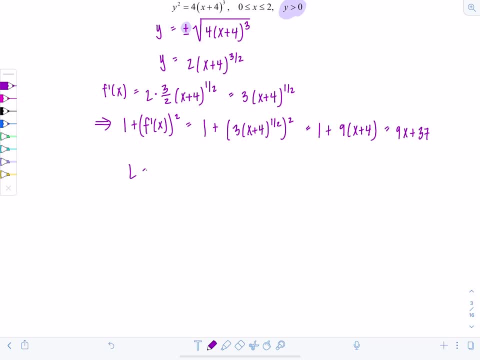 All right, And now we're ready to roll. So arc length is gonna equal definite integral. Okay, So arc length is gonna equal definite integral. They gave me the limits right here, From zero to two, And then I have square root of nine x plus 37 dx. 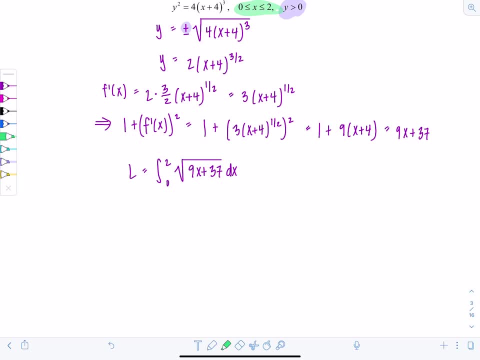 Okay now, hopefully at this point you don't need to do a u sub. You can just imagine if you were to u sub and let u equal nine x plus 37, du would be nine dx, So you would have a one ninth in the integral. 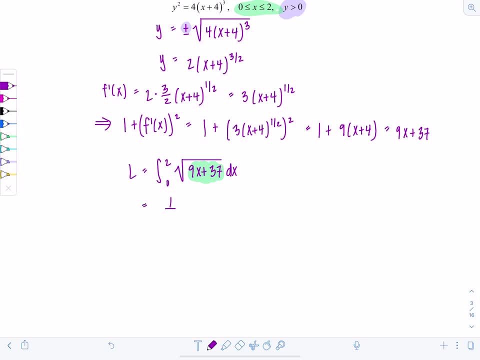 So let's just take care of that. And then let's see here: So nine x plus 37 is raised to the one half power. If I add one, that's three halves. And then I need to divide by the new exponent. 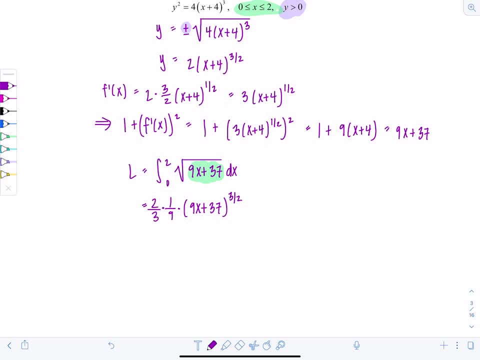 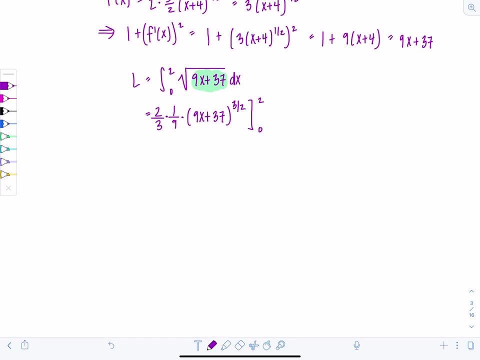 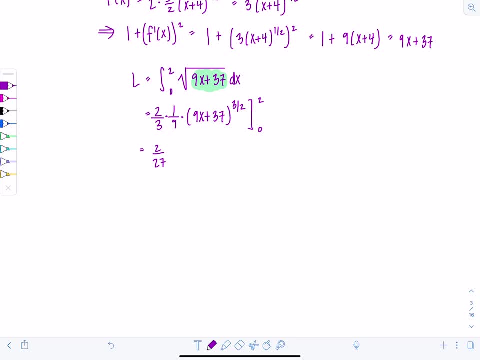 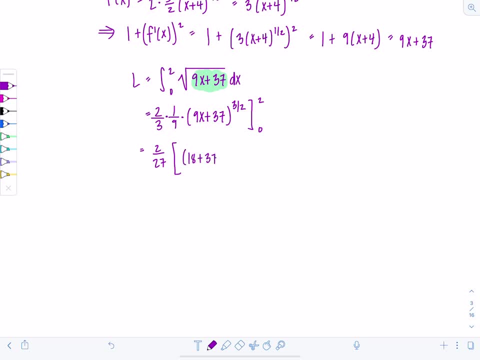 So nine times two, that's gonna be 18 plus 37 to the three halves. And then, be so careful, zero plus 37 is still 37 to the three halves. And then, be so careful, zero plus 37 is still 37 to the three halves. 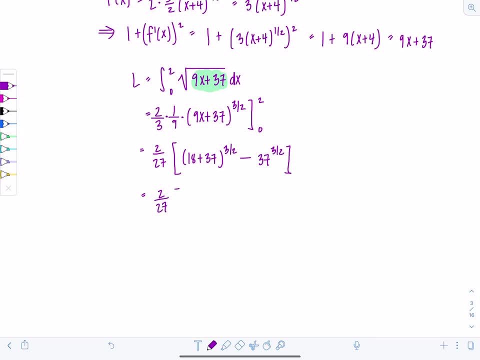 All right, so we have two over 27 times this is 55 to the three halves minus 37. times. this is 55 to the three halves minus 37.. 37 to the 3 halves, and then we can just rewrite our final answer: 2 over 27 times 55, rad 55. 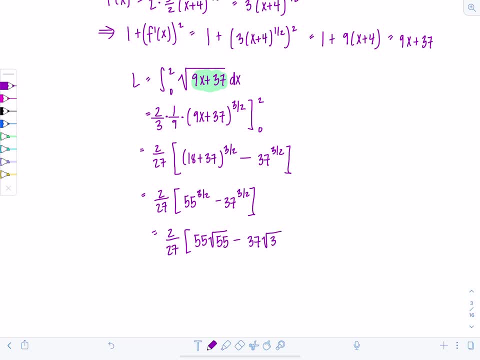 minus 37, rad 37 and nothing else distributes or cancels, so we'll just leave it like that. all right, how was that? not too bad, right? normally these integrals aren't too crazy like the ones in the previous unit. um, they're just like a few classic ones. so this is one of. 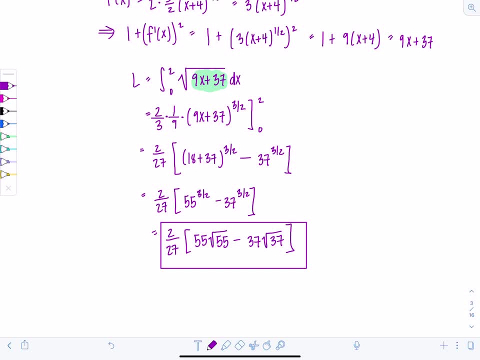 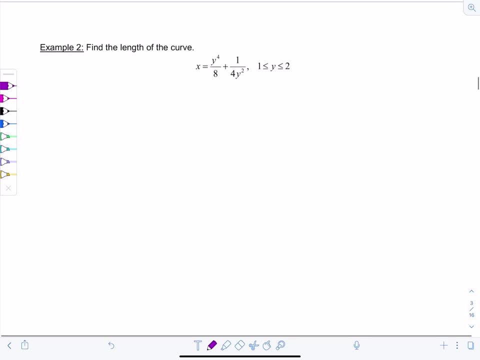 them. and the next one i'm going to show you. you need like this little slick factoring maneuver, but then, once you see it again, you're like: oh, that old problem. so here we go. find the length of the curve. this time x is a function of y and it's y to the fourth over eight plus one over four. 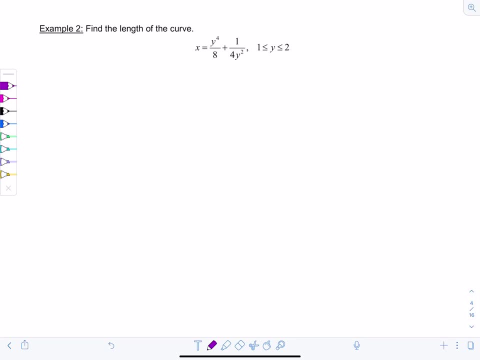 y squared y is from one to two. i'm going to rewrite it in derivative friendly format, as you. this is one eighth y to the fourth, plus one fourth y to the negative second. so we'll be ready to differentiate it and in this case, since x is a function of y, the arc length formula we're. 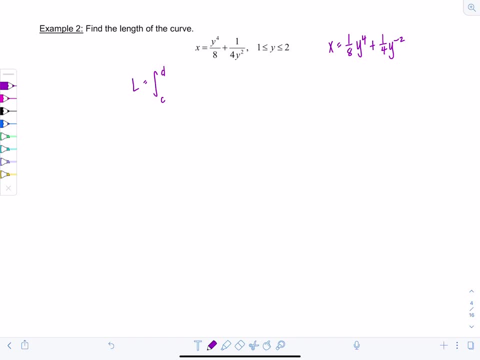 going to use is the integral from c to d of the square root of one, plus dx dy squared dy. all right, so let's take the derivative, clean it up as much as possible, and then we'll start integrating. so here we have dx- dy equals. so now i'm going to differentiate this guy. 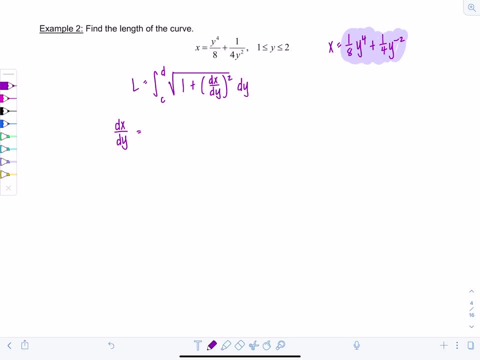 so one eighth. y to the fourth, that's going to be four over eight y cubed minus two over four. y to the negative third, which is one half y cubed minus one half y to the negative third. all right, beautiful. now remember what i integrate is one. 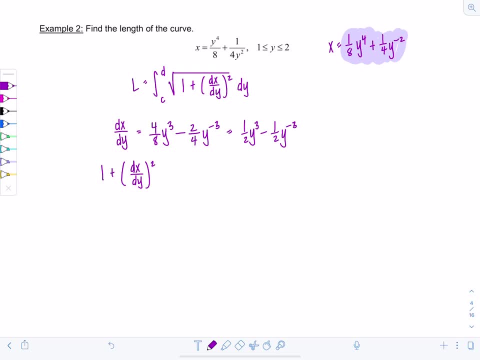 plus that derivative squared. so let's do all the prep work now. so one plus. now i'm going to square this quantity. so remember you're going to square the first term. so you have one half y cubed squared, minus two times the product of the first. 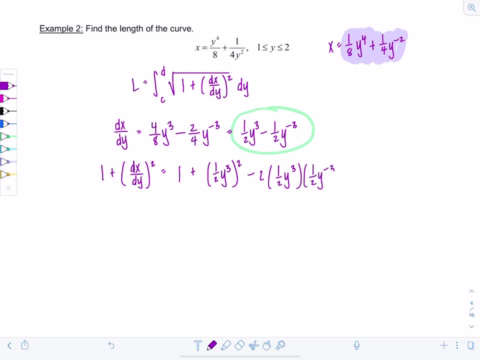 and second terms: one half y cubed, one half y to the negative third plus then i square the last term, one half y to the negative third, squared. i'm really breaking it down. i don't ever do it this way because i know the pattern and i can go more quickly. but this is just to show you, guys, for the 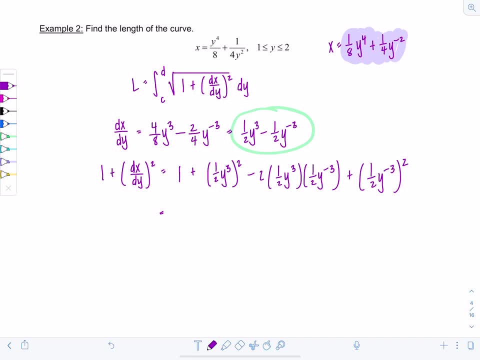 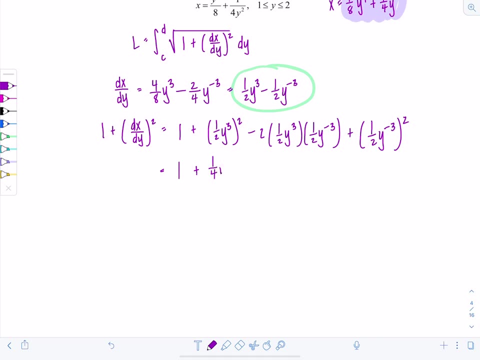 first time. all right, look at this. so we have one plus. if i square one half, y cubed, that's one fourth. y to the sixth minus. now notice the two and this one half cancel. and then we add our exponent. so y to the third and y to the negative third. that's going to give us y to the zero. so y's are gone, they cancel. 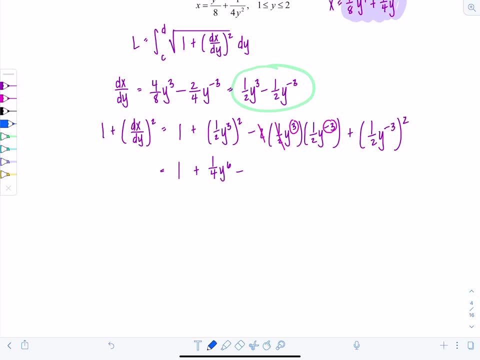 out completely. all i'm left with is a one half from that term, plus, if i square the last term, that's one fourth y to the negative sixth. so this is what i get when i squared the derivative. okay, anything else you notice we can do. well, i see this one and this negative one half, let's. 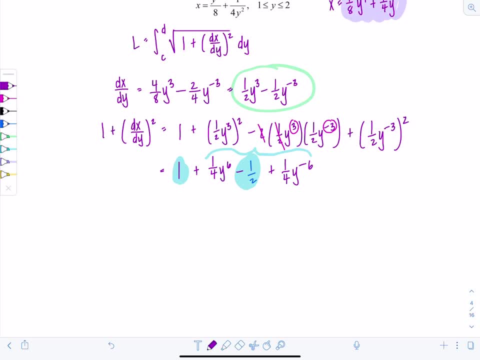 combine them, okay, and i'm gonna write it now as one fourth y to the sixth, plus one half, plus one fourth y to the negative sixth. so all of this is supposed to go underneath the radical. but remember, you want to make life as nice as possible for yourself, so is this a nice quantity to take the square root of? 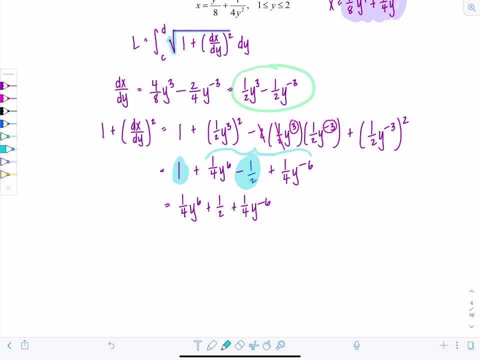 no, i don't. i don't think it is, and i want you to notice something: here's the big, here's the big trick to this problem. when we took this expression right here, the derivative one half y cubed minus one half y to the negative third, and we squared it and cleaned it up, we ended up with one fourth y to 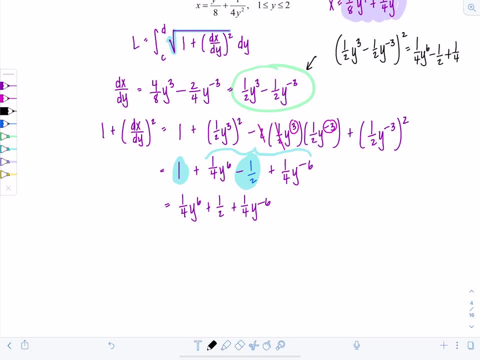 the sixth minus a half, plus one fourth y to the negative sixth right, we ended up with this expression and now, after i added the one, i have this expression down here, we'll compare this with what we got when we multiplied out the derivative, when we squared it. 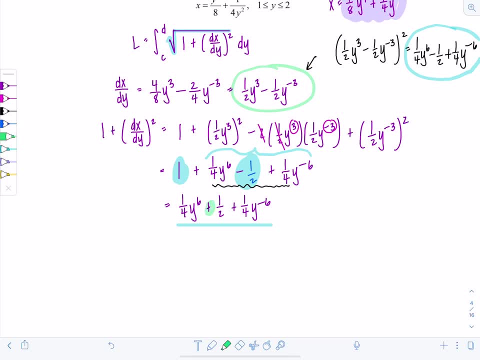 but the only thing that's different is i have a positive one half here and this was a negative one half, which means this is going to factor very similarly to how dx dy was factored before we squared it. so this is going to be one half y cubed plus one half y to the negative third squared. 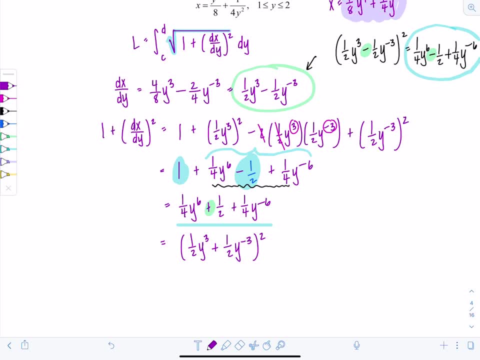 and now we're ready to put it all together, because i can easily take the square root of this and then anti-differentiate. did you guys see that slick factoring? okay, this is a classic problem, so the equation will change a wee bit, but the idea is the same. you always end up with that negative one, half. you add the one, you get a. 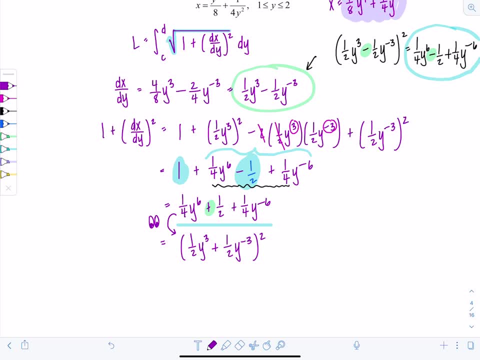 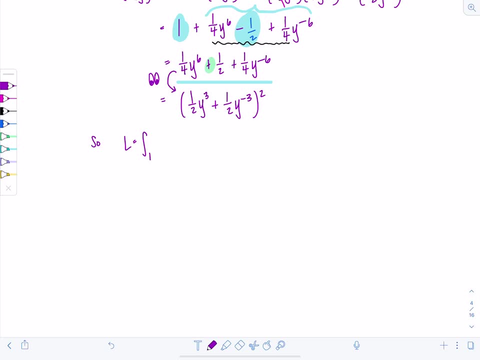 positive one half and then you refactor with the plus. i kid you not okay. so putting it all together, the arc length is equal to the integral from one to two. i have the square root of 1 half y cubed plus 1 half y to the negative third squared dy. 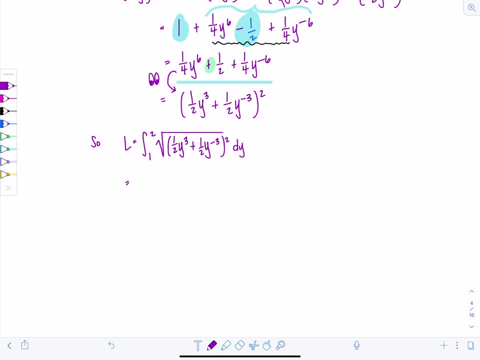 which all cancels out right the squared and the squared root. so we have 1 to 2, 1 half y cubed plus 1 half y to the negative third dy. all right, you know, we can take this 1 half outside, so let's do it. so I have 1 half times now, let's. 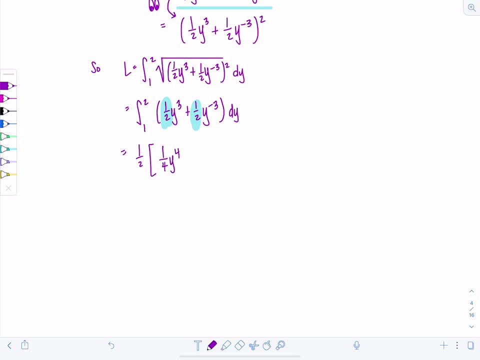 anti-differentiate. this is going to be 1 fourth y to the fourth. add 1 to negative 3, it's negative 2, so I'm going to divide by that. so negative 1 half y to the negative second. evaluate this from 1 to 2, and now I have 1 half times. let's see. 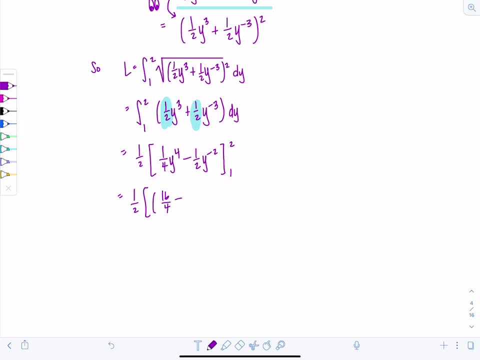 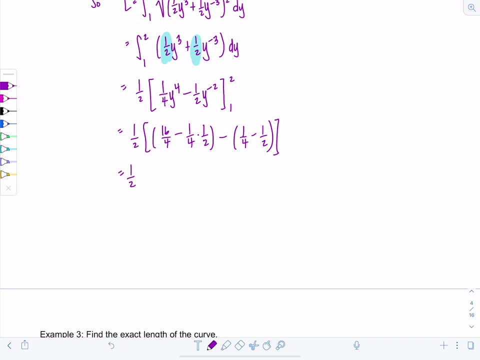 here. so 2 to the fourth, that's 16 over 4 minus 2. to the negative second, that's 1- fourth, and I still have the 1 half minus. if I plug in 1, I have 1 fourth minus 1 half. okay, so this is 1 half times 4 minus 1. eighth minus 1. 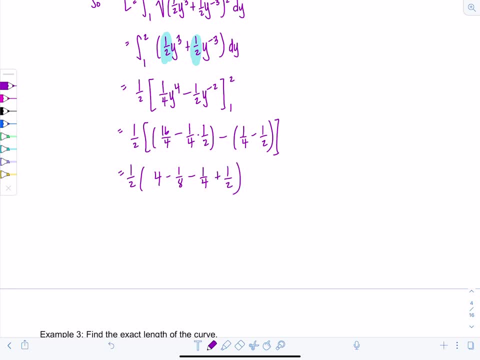 fourth plus 1 half yay fraction. so this is 1 half times common denominators 8. you should end up with 33 over 8. so this is 33 over 16. whoo, all right, I kid you not, you're gonna run into that little classic factoring. 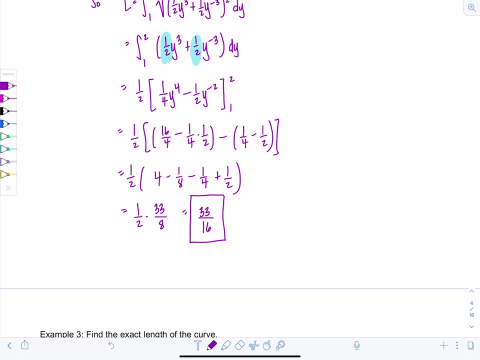 problem so many times. if you open any old calc book it's in there. just the exponents might be a bit different, okay, but now you know. now you know the trick, you can Wow all your friends. I got one more example for you. are you guys ready? 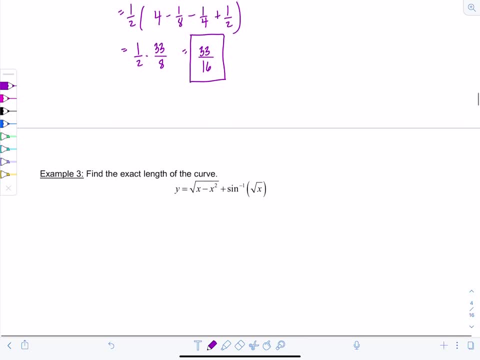 here we go. find the exact length of the curve. y equals the square root of X minus X squared plus sine inverse of radix. what in the world? they didn't give us limits. that means we have to figure out the domain of the function and just use that. 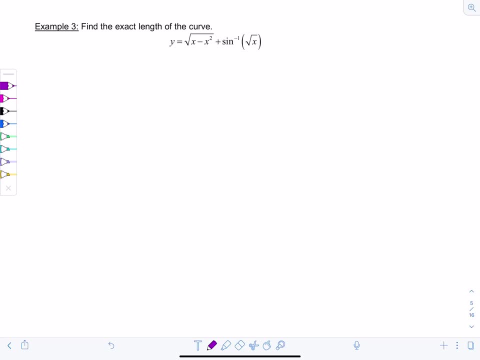 domain to give us our limits of integration. so let's see here. I have a radical function with an even index. that means the radicand, or the stuff underneath the radical, has to be positive. so X minus X squared has to be greater than or equal to zero. 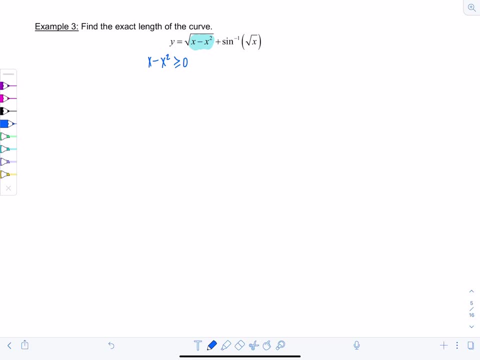 how do you solve a quadratic or higher order inequality? by finding the zeros and using test points. so X times 1 minus X has to be greater than or equal to zero. that means on the number line. then I list the zeros 0 and 1 and test each. 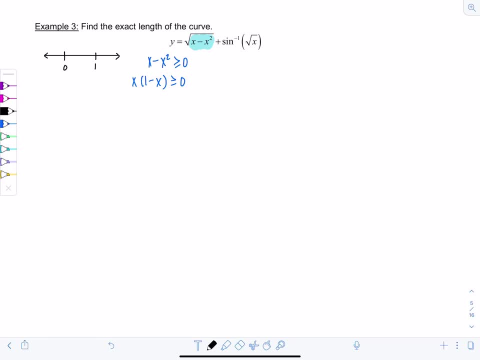 interval. so if I pick something smaller than 0, say negative 1 and I substituted in negative 1, this would be negative, this would be positive, so their product would not be greater than or equal to 0. so nothing in that interval works. if I pick something between 0 and. 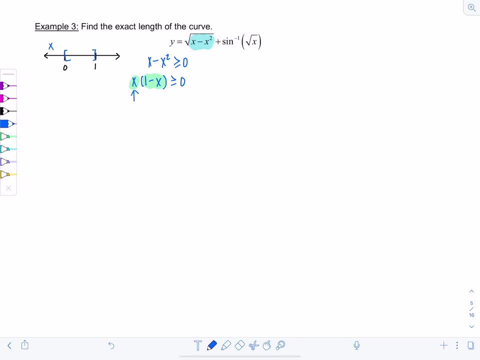 1 like 0.5. that would be positive. that would be positive. so the product is positive. so anything in this interval works. and then greater than 1 won't work either. similarly, sine inverse of rad X: again X has to be greater than or equal. 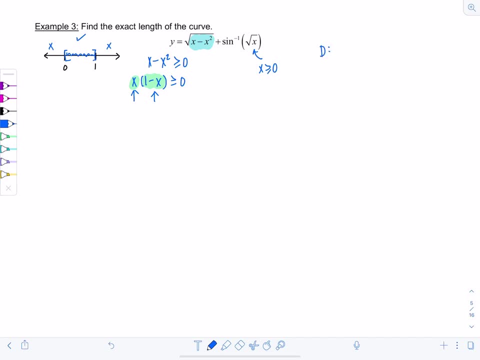 to zero because of that radical. So the domain for f of x or y of x is the interval from zero to one. So I'm going to use those as my limits of integration, because the function or the curve only lives there. That's its domain. There's no other x values for which it's defined. So if they're asking for the length, 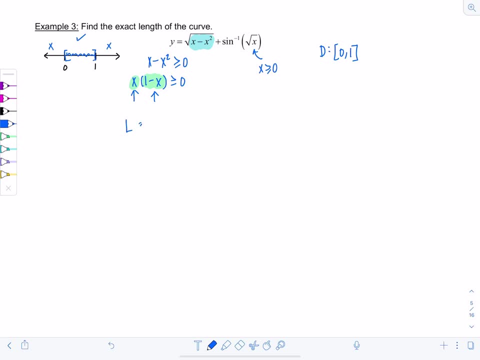 those are my limits. So the arc length is going to be the definite integral from zero to one square root, one plus dy dx, squared dx. So now let's go ahead. take the derivative. Okay, so dy dx, If I differentiate rad x minus x, squared, anytime you take the derivative of. 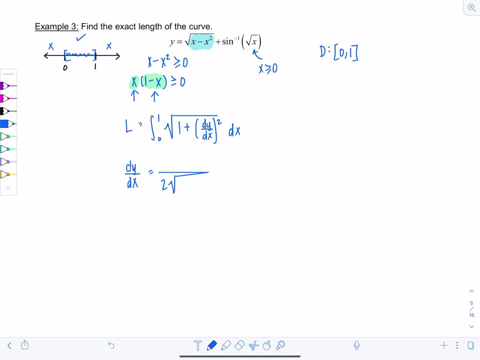 the square root, you end up with two: and the original radical expression in the denominator, And then by the change of the derivative you get the derivative of the denominator, And then by the change of the derivative you get the derivative of the denominator, And then by the 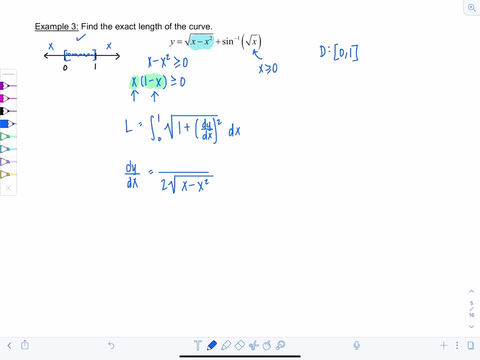 chain rule. you can just multiply by the derivative of the radicand, or x minus x squared in the top, So that would be one minus two, x plus, and then derivative of sine inverse of rad x, So it's going to be one over square root, one minus radical x squared, So that just becomes x. 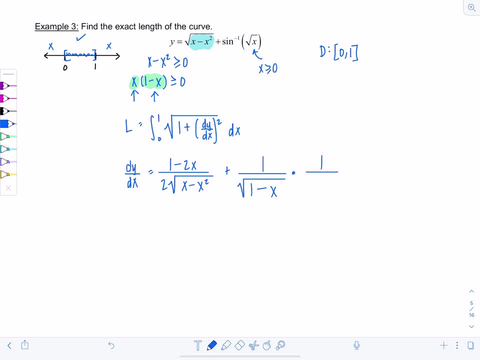 And then by the chain rule, I have to multiply by the derivative of rad x, which is one over two rad x. Well notice, I actually already have a common denominator. Someone loved us when they wrote this problem, My goodness, because rad x minus x squared is x times one minus x. 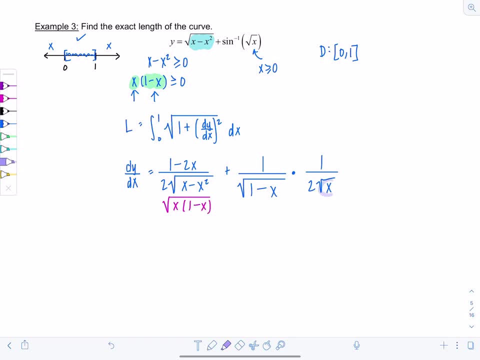 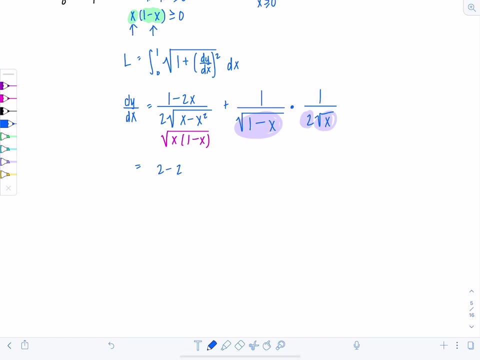 which is exactly what we have over here: Rad x, rad one minus x, and we even have that two, So we can already add the numerators together. This problem is a dream come true. I have one minus two x plus one times one, So that's two minus two x over two rad x times rad one. 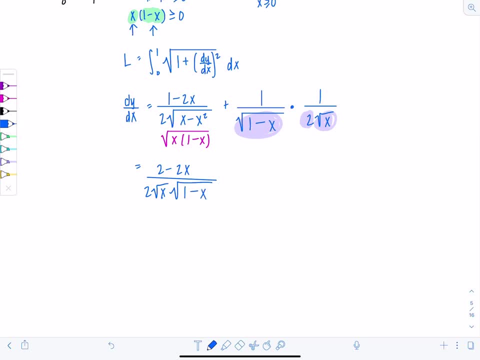 minus x. Can we clean this up? Yes, Okay, in the numerator I can factor out that two, And then I have one minus x over two rad x, rad one minus x, So that's two minus two, x plus one times one, So that's. 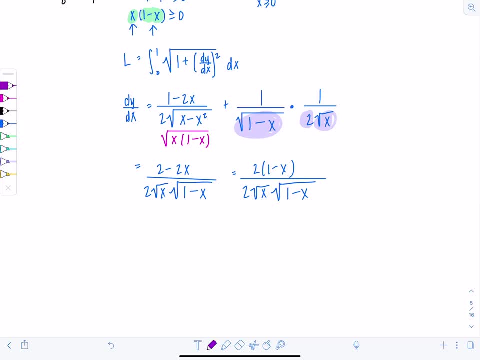 one minus x. So check this out. The twos cancel and the rad one minus x is gone. And instead of one minus x in the numerator now I have rad one minus x, Lovely. So this equals square root of one minus x over x. That's the derivative. Okay, well, what do I integrate? One plus the. 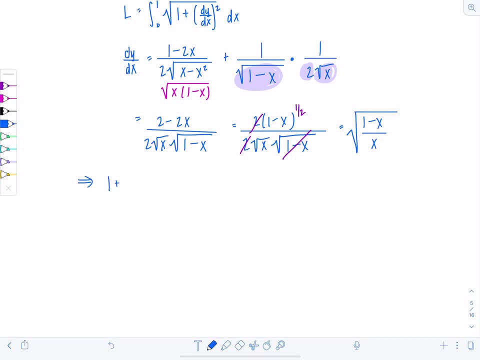 derivative squared, So that means one plus dy. dx squared is one plus. if I square this guy, the radical is gone. So I just have one minus x over x. Let's add them together. Common denominator is going to be x, So one becomes x over x. So I have x plus one minus x over x. 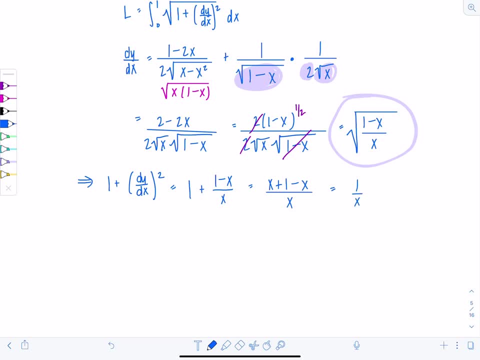 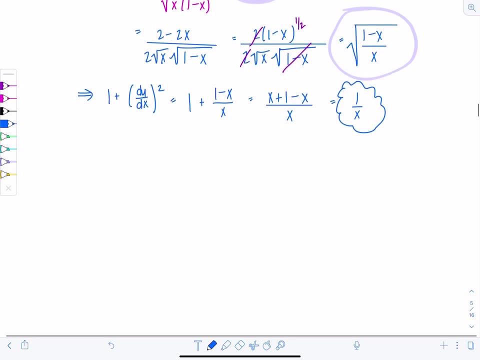 which is just one over x. Wow, this cleaned up big time right. It's like extreme makeover. So the arc length L is equal to definite integral zero, to one square root of one over x dx. Now take a look at this guy. Is something jumping out at you? I hope so. This is an 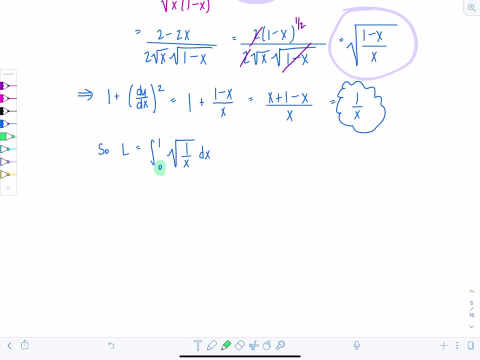 improper integral. If you forgot, it was just the previous video, Video number seven, Because zero is not in the domain of the integrand. So what do we do? We rewrite it as a limit. So I'm going to write this as the limit as t approaches zero from the right, because it's the lower limit. 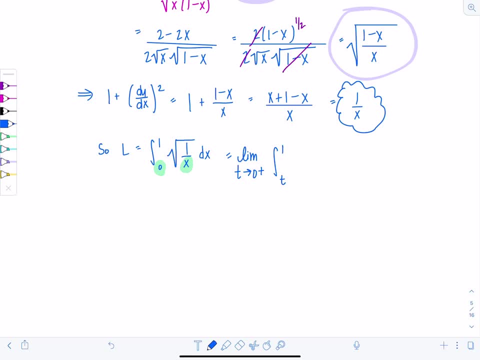 Integral from t to one- This is one over rad x, or same thing as x- to the negative one, half dx. I just like to rewrite it that way, so I'm ready to anti-differentiate. So now we have the limit as t approaches zero, from the right Anti-derivative of x to the one. 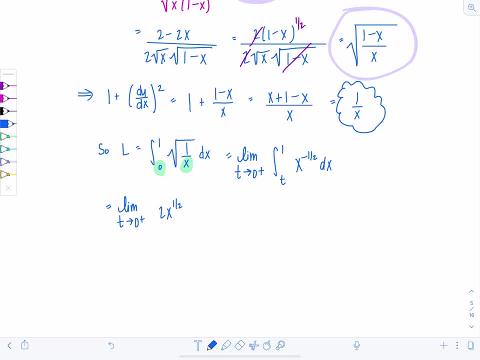 half is going to be two times x to the positive one half. I'm evaluating that from t to one. So this is the limit. t approaches zero. from the right, Plugging in the limits of integration, you're going to have two times one. 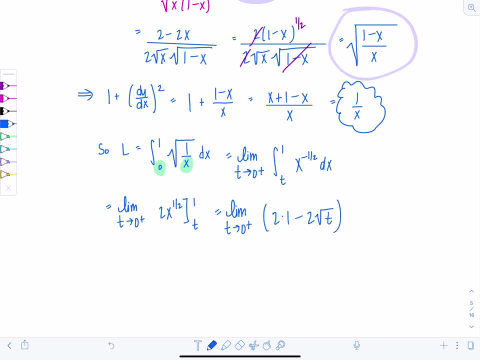 Minus two rad t t is approaching zero from the right, So this whole term is just going to go to zero And I am left with two. So that is the length of our curve. We made it All right. so that concludes the lesson on arc length. Believe it or not, a lot is going to build. 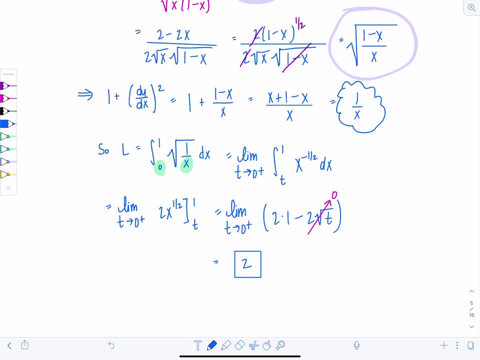 on this formula in calc two and even in calculus three. So make sure you do not forget the arc length formula, And I hope you enjoyed the lesson. Please give the video a thumbs up. subscribe if you haven't already. and next we're going to look at the surface area.